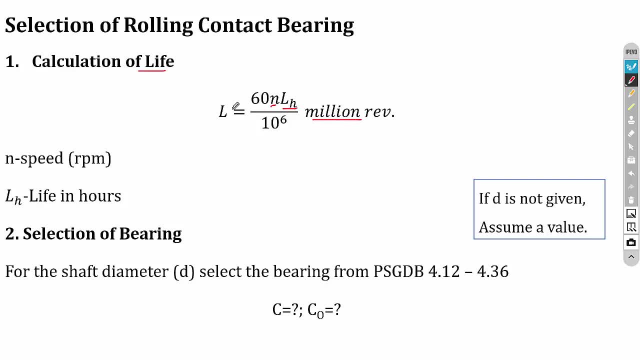 So this is the formula to calculate the life, or to convert the life in hours into life in million revolution. So this equation is not there in the data book, So you have to memorize this. So L is equal to 60n Lh divided by 10 power 6.. So here n is the speed in rpm that will be given, and Lh is life in hours. So that is also a given data. 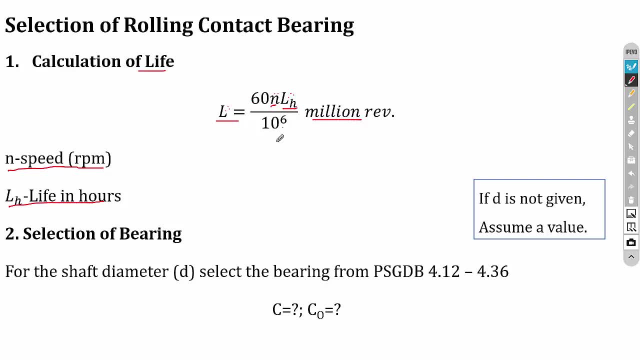 So by substituting n and Lh you can calculate L in million revolution. So this is the first part. The second part is minerals. So N is the melting point, The second part is the temperature. The third part is the electronimate coil. 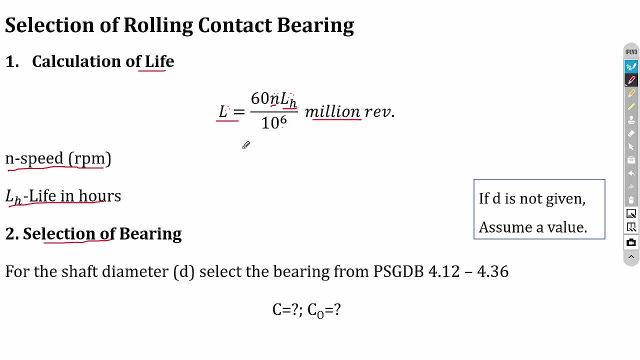 step is selection of bearing. so once after calculating the life in million revolutions by considering the shaft diameter D, you can select a suitable bearing. okay, so we have the standard bearings from PSG data book, page number four, point one, two, two, four, point three, six. okay, so in that you can select a. 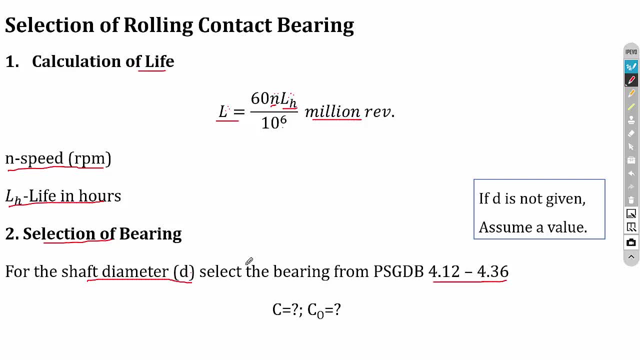 suitable bearing for your application based on the shaft diameter. okay, so in some of the problems the load will be given but the shaft diameter will not be given. okay, but without shaft diameter we cannot select the bearing. so if the shaft diameter is not given, then you have to assume a shaft diameter and you 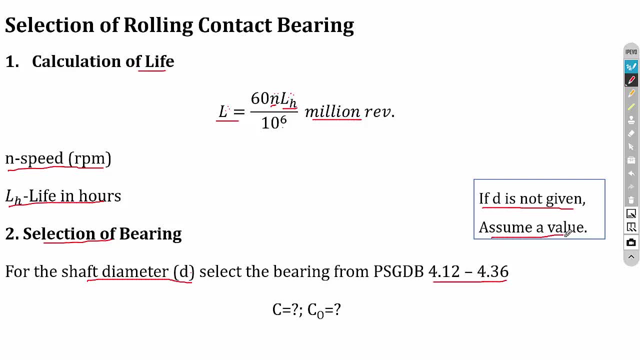 can select a suitable battery case. so if the shaft dia is given, then you can use it our, otherwise you can assume a suitable shaft diameter. okay, so after calculating the, after selecting the suitable bearing, then you can write the system. or you write two words: a machine, while customizing the Nobel, isn't it real? 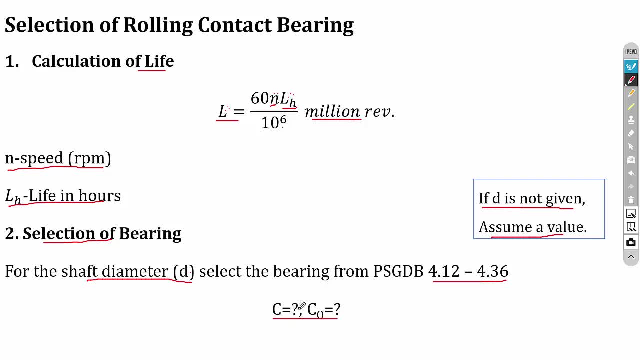 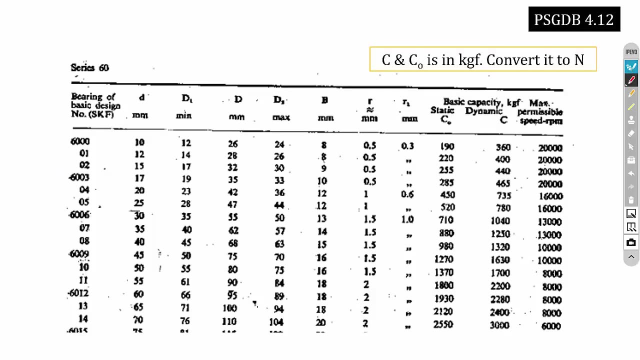 C and C0 of the selected bearing. So these two data's will be in the data book. So C means it is the dynamic load carrying capacity and C0 is the static load carrying capacity. So this is the chart to select the suitable bearing. So actually we have different charts. So we have series 60, we have series 62 in page number 4.13 and we have series 63 in page number 4.13,. no, I mean 1.4.. 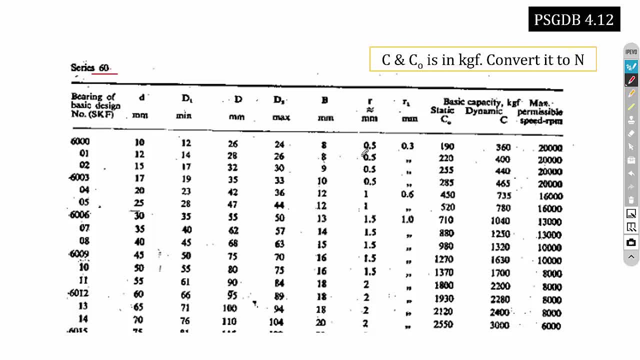 So series 60 means it is a light duty bearing, series 62 means it is heavy duty bearing. So based on the load recruitment we can select the bearing. So here we have to consider the shaft diameter. that is small d So for example, if my shaft diameter is 50, then here it is 50 mm and the selected 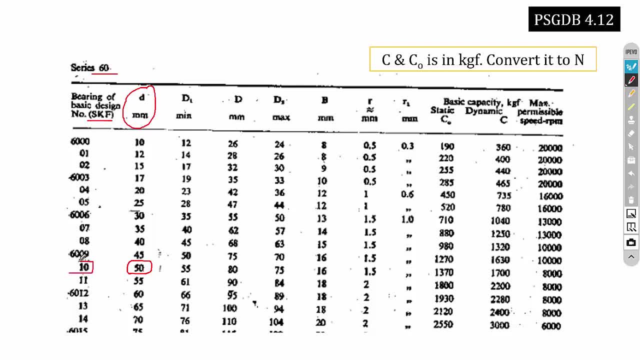 bearing is SK of 6010.. So it is 6009, so it is 6010. and for the 6010 bearing the C value is 1700. it is actually in kgf, So you have to convert that kgf into Newton. 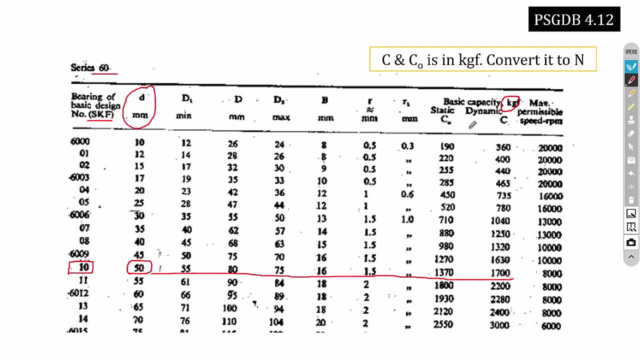 So you can multiply 10 with that, So it is 17000 Newton. that is dynamic load carrying capacity C and the static load carrying capacity is C0.. It is 1370 kgf or otherwise it is 13700 Newton. So based on the shaft diameter you can select the bearing. So the selected bearing is serial. 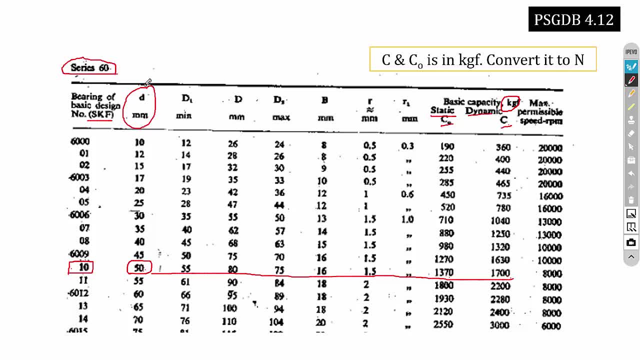 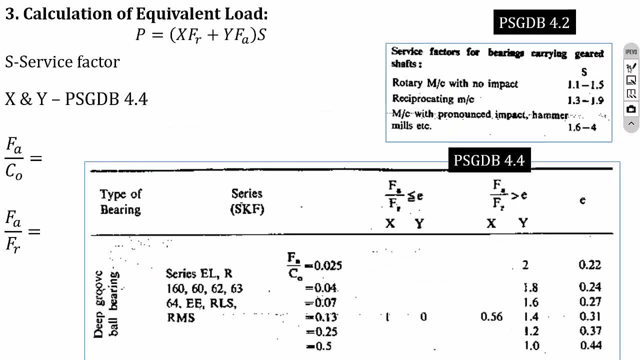 60. So series 60 is actually a deep groove ball bearing and the selected bearing number is 6010.. So now we have selected the bearing, Now we have to check whether the selected bearing is suitable for our application or not. So for that we have to calculate the equivalent. 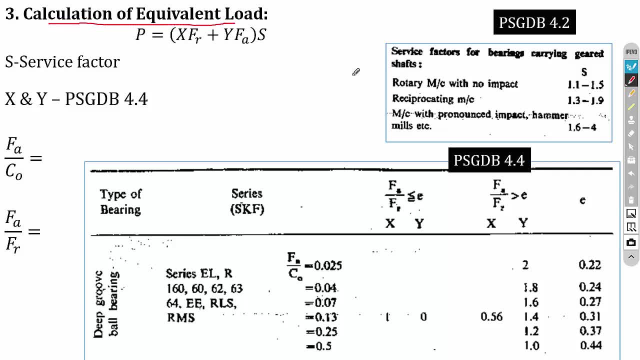 load, So actually in rolling contact bearings. so the rolling contact bearing is designed to withstand two kind of load. One is radial load and the other one is axial load. So axial load means it lagged parallel to the axis of the shaft. In case of radial load it lagged 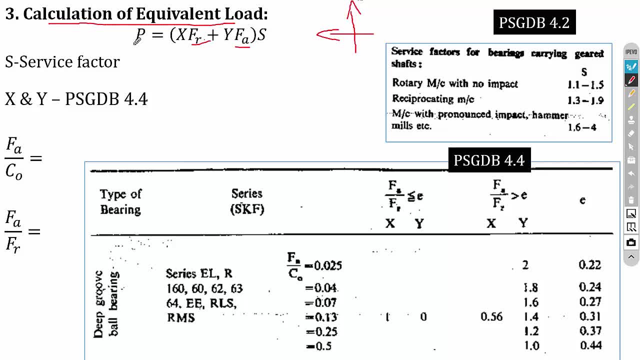 perpendicular to the axis of the shaft. So this P is the equivalent load So it has. so it is the combination of both radial as well as the axial load. So the equation is: P is equal to X into FR, plus Y into FA into S. So here FR is the radial load. 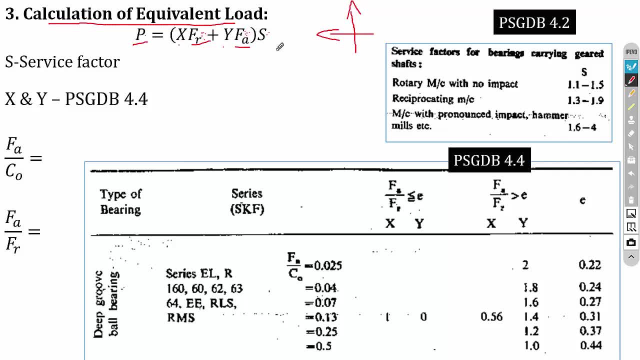 It is a given data. FA is axial load, Then S is the service factor. So this equation is there in data book, page number 4.2.. Also, you have the service factor values on the same page. So for rotary machine with no impact, the S should be between 1.1 to 1.5.. For reciprocating: 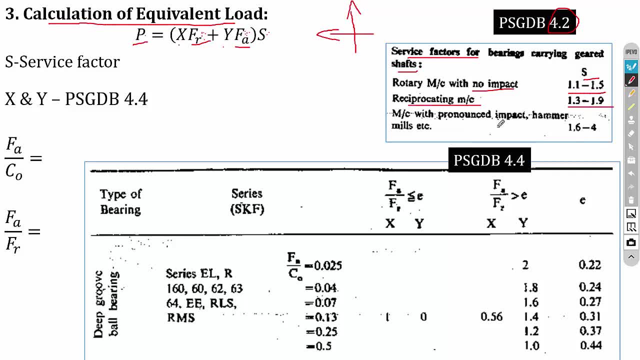 machine, it should be between 1.3 to 1.9.. And for rotary machine with impact then it should be between 1.6 to 4.. So you can select the S value from the data book, Then the X and 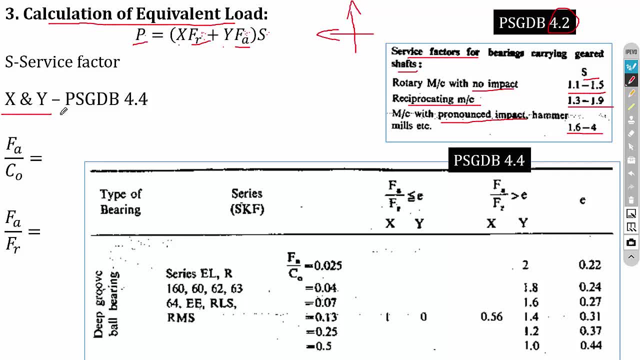 Y value. So X and Y value, actually we have to select from the chart that is available in page number 4.4.. But to select the value we have to calculate the two parameters. So based on these two only we have to select the value. So first one is FA by C0.. So you, 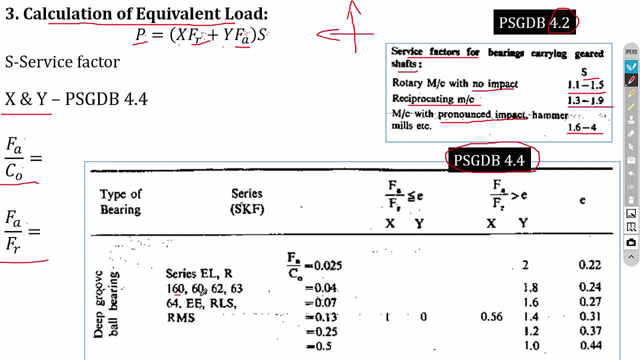 can see that Series 60, 62,, 63 and 64. We have a series of X and Y values, So this values depends on this FA by C0. So first we have to calculate the FA by C0.. FA is the axial load, that is. 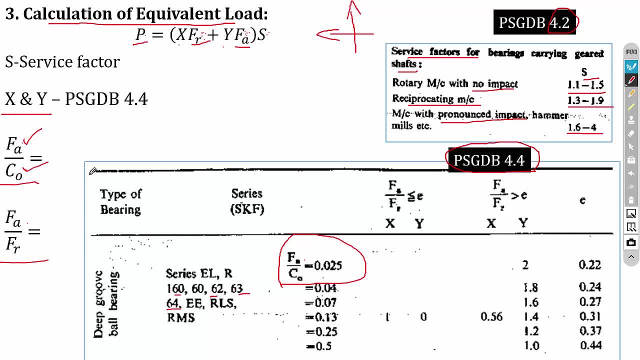 given in the problem, and C0 is the static load carrying capacity, So that is the property of the bearing, So that we have selected earlier, So based on the FA by C0, for example, if my FA by C0 is 0.1.. 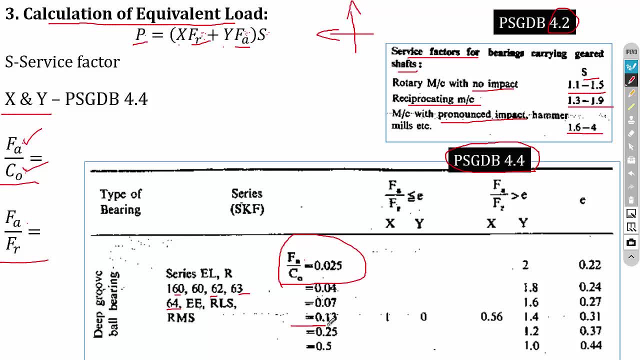 So that is the property of the bearing, So that we have selected earlier. So based on the FA by C0, for example, if my FA by C0 is 0.1, then I can select the next standard value, That is, FA by C0 is equal to 0.13.. So for 0.13, I have two values, of X and Y. 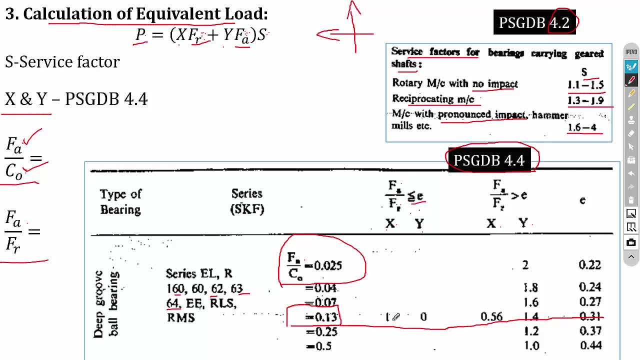 So if the FA by FR is less than E, then X is 1 and Y is 0.. If the FA by FR is greater than E, so E is given here. So for the FA by C0 is 0.13, then I can select the next. 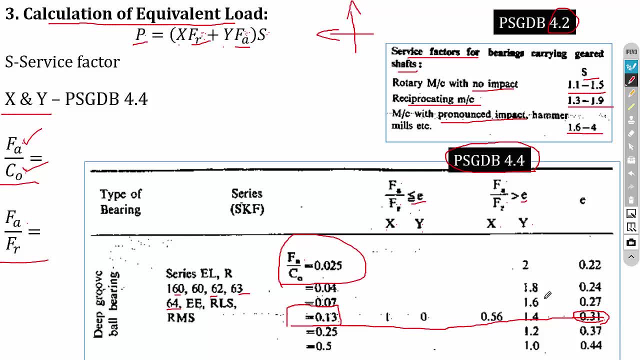 standard value. So that is very important. The selection of x and Y is very important, So remember that. First you have to calculate the FA by C0 value. So here the calculated value is 0.1, that is the why I selected the next value, that is, 0.13. 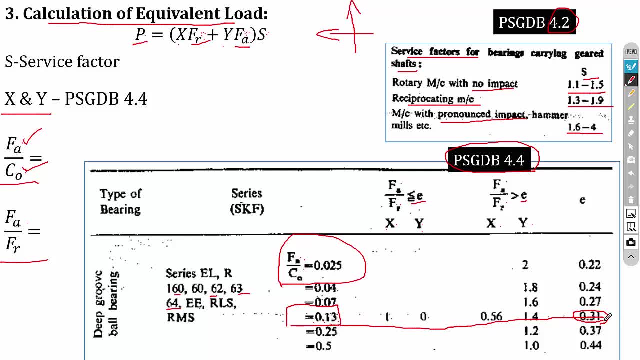 So for FA by C0 is 0.13, the E value is 0.31.. So for E value is 0.31, I can calculate the F A by F R. So if my F A by F R is less than E, then X is 1, Y is 0.. If my F A by F R is greater than E, then my X is 0.56 and my Y is 1.4. 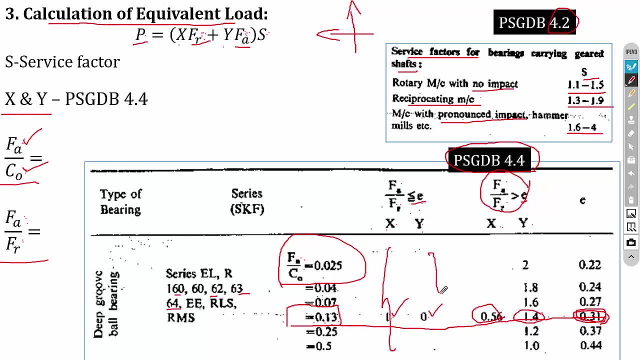 So here, for all this value, the X is 1 and for all this value the X is, I mean Y is 0. And here, for all the values of F, A by C naught, the X is 0.56.. Only the Y value is going to vary. So for calculating the X and Y value, these two things are very important. 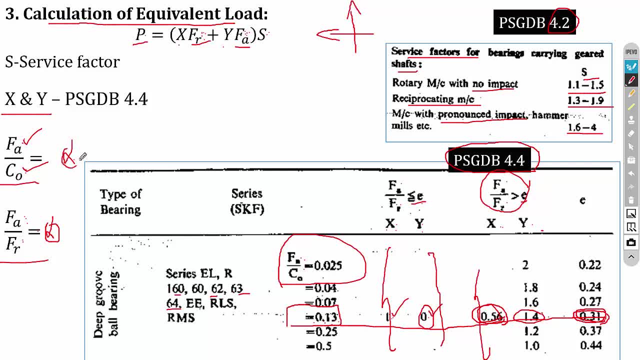 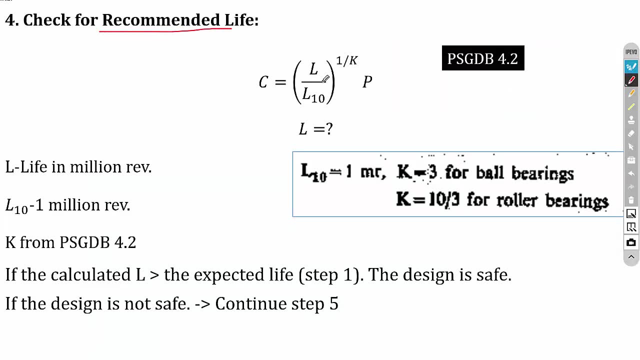 So the F A by C naught as well as the F A by F R, So now you can substitute everything. You can calculate the equivalent load. So once after calculating the equivalent load, we can calculate the life of the bearing. So you can calculate the life of the selected bearing. 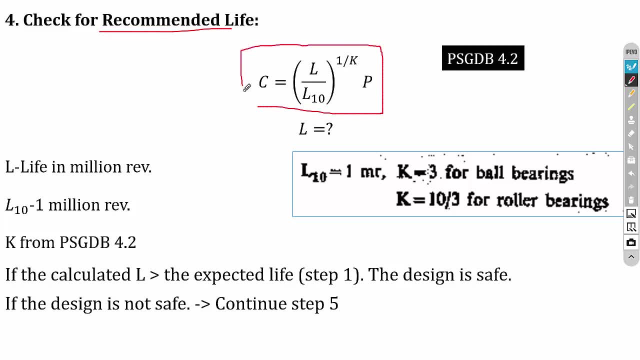 So this is the equation to find the life of the selected bearing. So this equation is there in the data book, page number 4.2.. So the equation is: C is equal to L divided by L10 to the whole power, 1 by K into P. 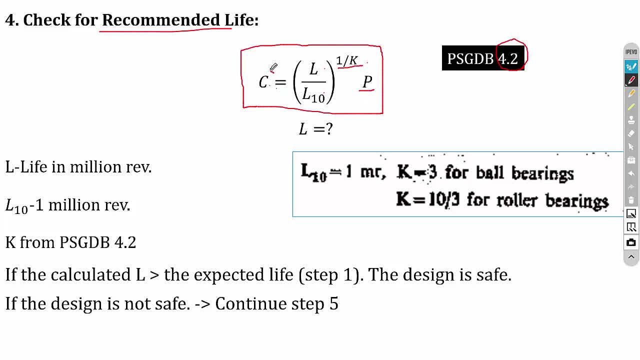 So here, the- Here C is the dynamic load carrying capacity, So that what we have selected from the data book P is the equivalent load L we have to calculate. So L10 is 1.. So it's a constant. So it is there in data book. L10 is equal to 1 and K is another constant. It depends on the nature of bearing. So this is also available in data book page number 4.2.. 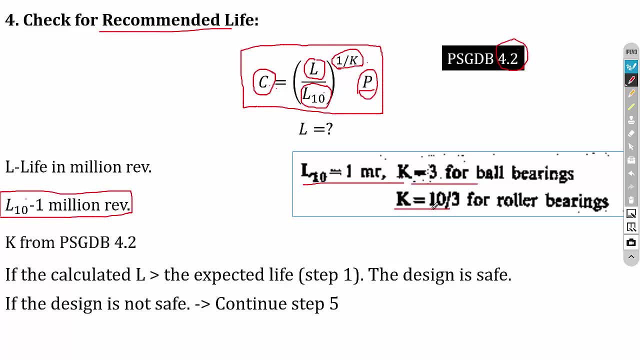 So K is equal to 3 for ball bearings and K is equal to 10 by 3 for roller bearing. So, based on your type of bearing, you can select the value of K, Then P you can substitute it. So finally, we have to calculate the L value. 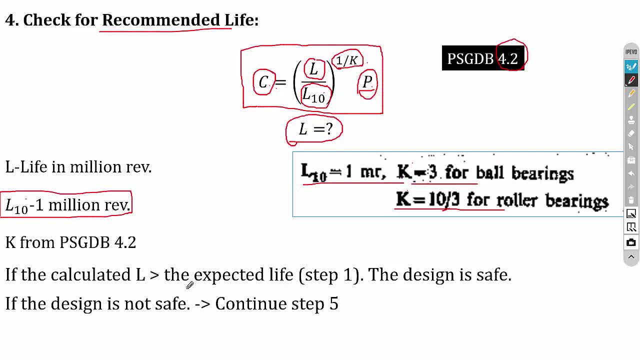 So previously in the first step we have already calculated and expected life. So this calculated- that is fourth step- L should be greater than the expected life. The expected life is given in the problem. The calculated L is the life of the selected bearing. So the selected bearing should satisfy the expected life. So if the calculated L, that is L calculated in step 1, is greater than L calculated in step 1, then the design is safe. 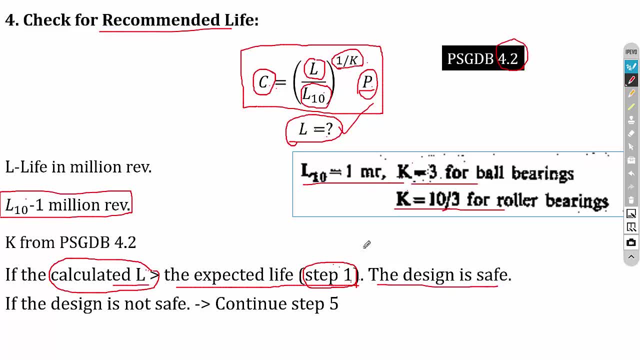 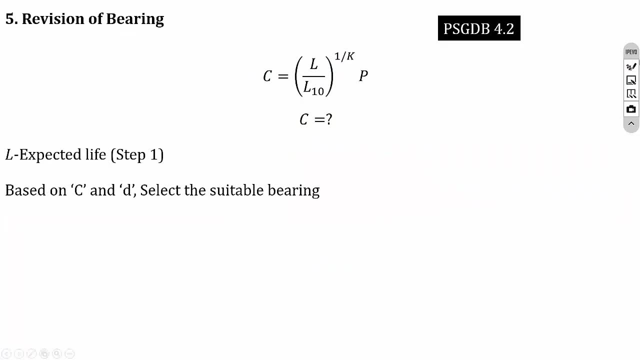 So this L should be greater than L calculated in step 1.. So or otherwise, the design is not safe. So if the design is safe, then you can conclude the problem. If the design is not safe, then you can move into the next step, That is, revision of bearing. 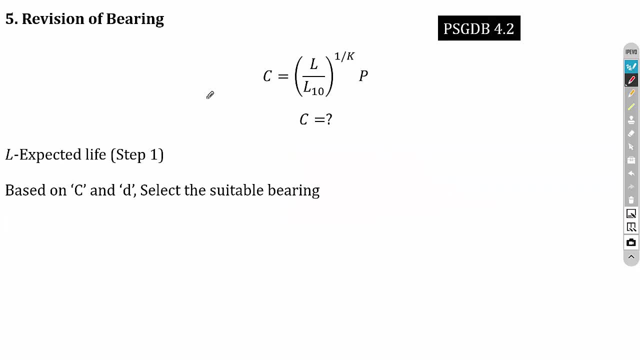 So, for example, the calculated L value is less than the expected life. So in that case I am going to calculate the expected dynamic load carrying capacity of the bearing So you can substitute the L value that is calculated in step 1.. So you should not substitute the L value from step 4.. 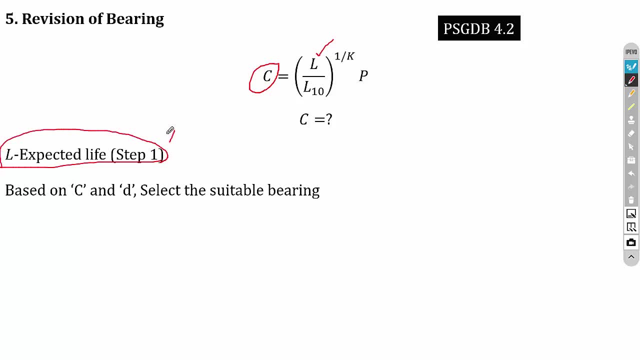 So you have to substitute the L value from step 1.. That is very important. And L10 is 1.. K is a constant. previously we have selected P, we have calculated and calculate the value of C. So now we have two values, So one is C. So previously we have only one data. 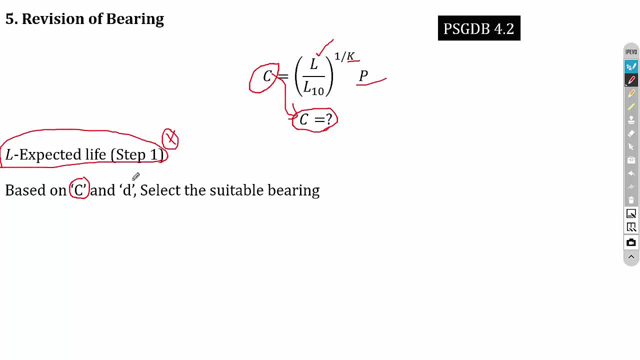 So that is why we have approximately selected the series, because you can select Either 60 series or 62 series or 63 series. But now we have two data- One is C and another one is D. So by having these two data's in our hand, we can accurately select the suitable bearing. 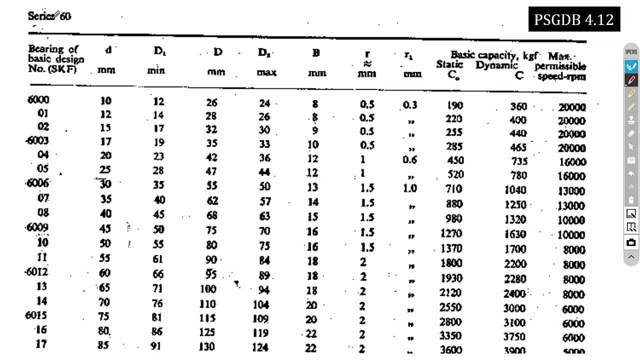 So I will show you how to select the bearing. So this is series 60.. So for series 60, and assume your shaft diameter is 50 mm, So this is 50 mm. This is the C value. So it is actually in kg. 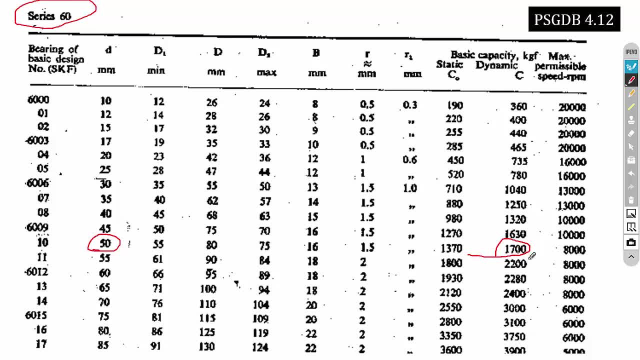 So this is the C value. So it is actually in kg. so if you convert it into newton it is around 17000 newton. okay, so if your c value is less than 17000, then you can select this bearing- okay or otherwise. you can move into the next page that. 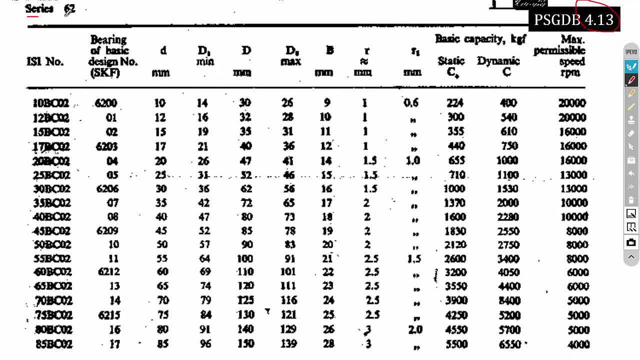 is page number 4.13, so the series is 62.. so here, if you look into the diameter 50 mm, then your c value is 2750 kgf, that is into 10, 27500 newton. so here, since it is a heavy duty, bearing the load, 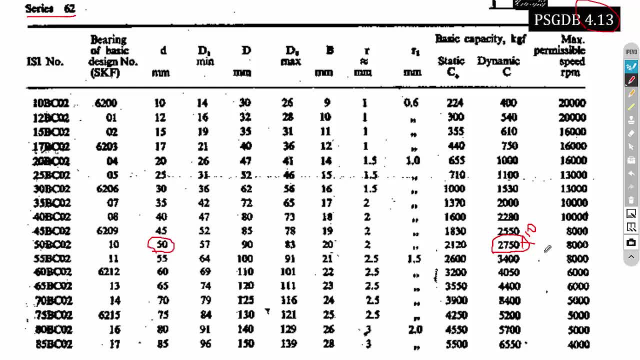 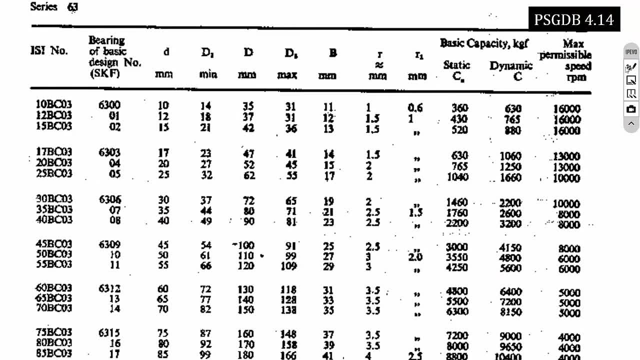 carrying capacity is slightly above the previous one. so further, if your expected c value is high, then you can move into the next series, that is 63 series. so here for 63 series and 50 mm diameter, your c value is 4800 kgf, that is 48000 newton. okay, so if your c value is 45000 then you can select this bearing. 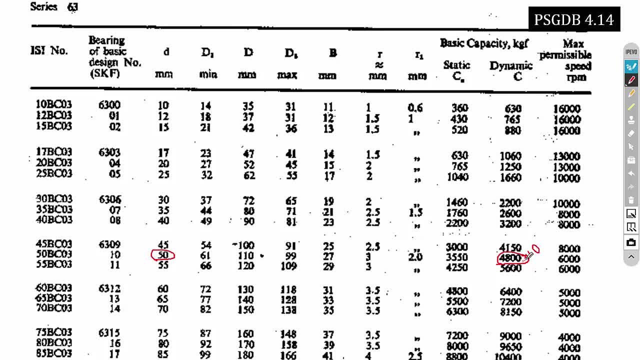 that is expected c value is 45000, then you can select this bearing. so, similarly, you have to turn the pages, you have to look into the various series and you have to select your suitable bearing. so in that case, if your load carrying capacity matches with this bearing, then your 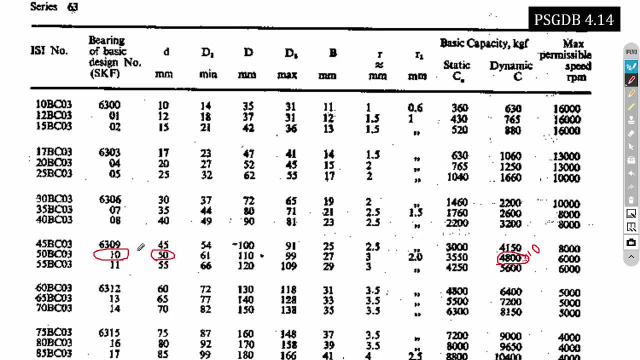 selected bearing is 6310 kgf. is 6310 kgf. okay, so it is not 6010 kgf, it is 6310 kgf, that is 63 and diameter 50. so at last you have to write that the revised bearing is skf 6310 kgf. 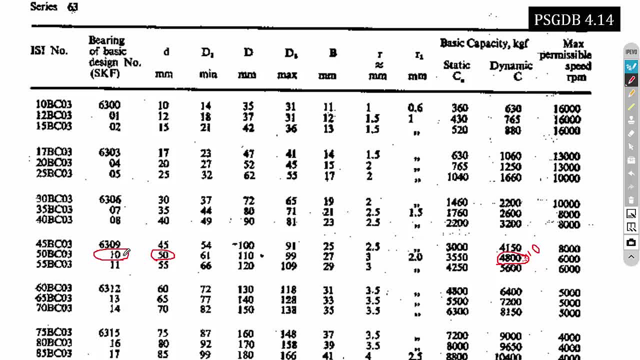 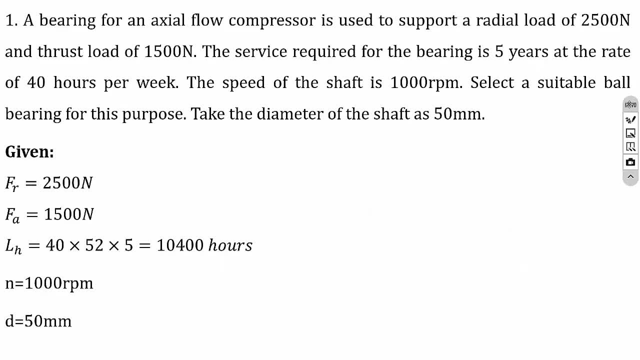 okay, so this is how design of selection of bearing goes on. so we will discuss a problem on that. baring for an axial bearing. we will training it, so when we will do that? baring for an Axial flow compressor is used to support a radial load of 2500N and thrust load of 1500N. 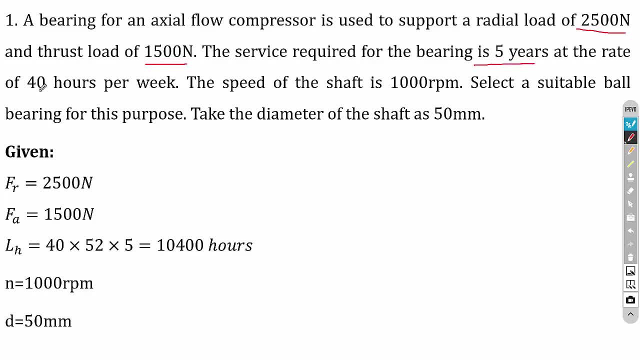 The service required for the bearing is 5 years at the rate of 40 hours per week. The speed of the shaft is 1000 rpm. Select a suitable ball bearing for this purpose. Take the diameter of the shaft as 50 mm. 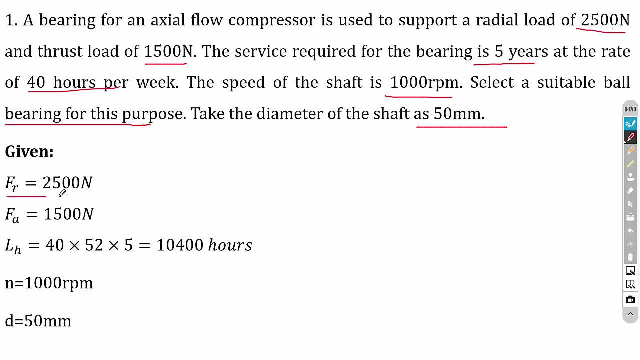 So we will write the given data first. The radial load is given as 2500N, The axial load is 1500N, Then LH. first we have to calculate. So actually the bearing is working for 40 hours per week for 5 years. 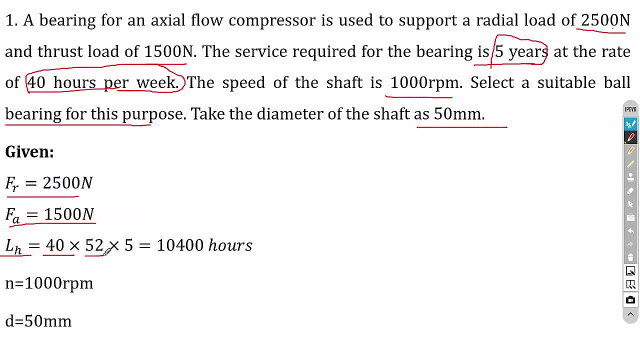 So 40 into 52.. So 52 for weeks, So 40 into 52.. So for 5 years totally. the bearing has to work for 10400 hours And the speed is 1000 rpm, So the shaft speed is given as 1000 rpm. 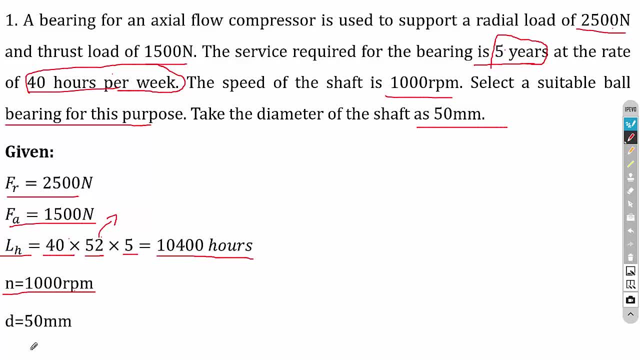 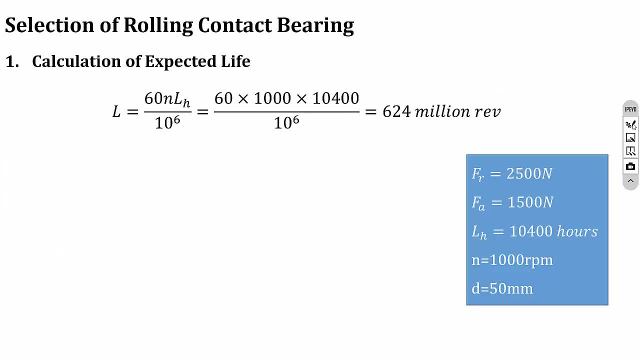 Select a suitable ball bearing for this purpose. The shaft diameter is given as 50 mm, So D is equal to 50 mm. So we will move into the selection procedure. The first step is calculation of expected length. The first step is calculation of expected length. 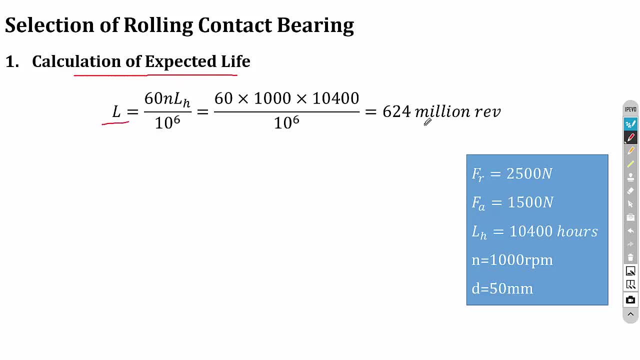 The first step is calculation of expected length, That is, we have to calculate L in million motor life, So that is L in million revolution. we have to calculate So the E иск ay 60n LH, divided by 10, power 6.. 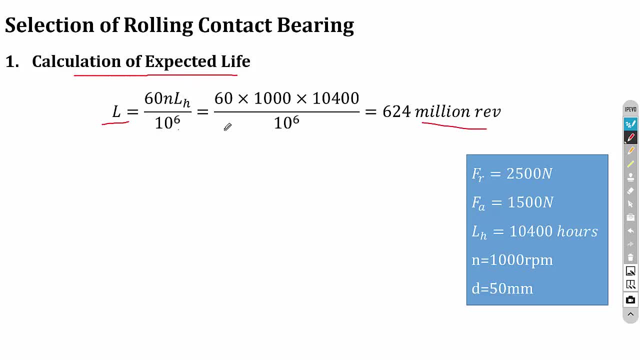 So 60 N is speed in RPM, That is 1000 RPM. So 60 N is speed in RPM, That is 1000 RPM, And LH is life in hours, That is 10,400 hours divided by 10 power 6.. 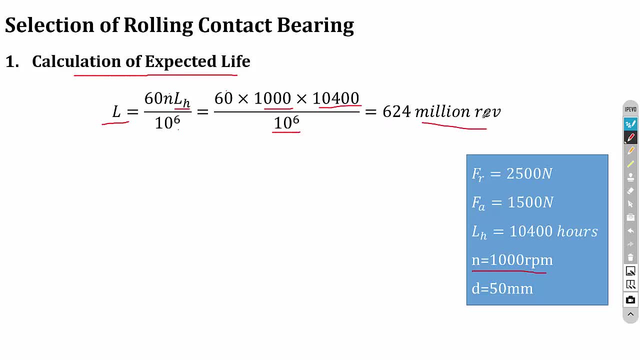 So L is equals to 624 million revolution. So this is actually the expected life on habían על Stokely Steel. So L is equals to 624 million revolution, expected life of the bearing. So actually in the problem the expected life is given. So in some of 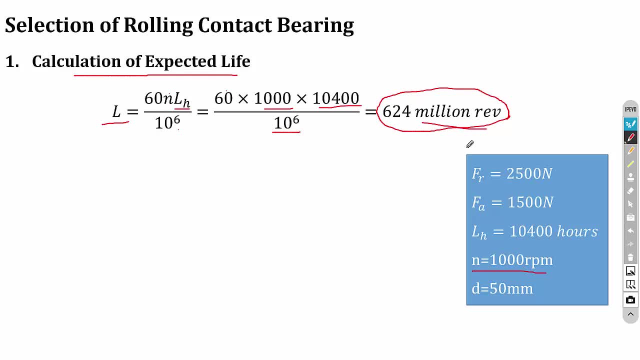 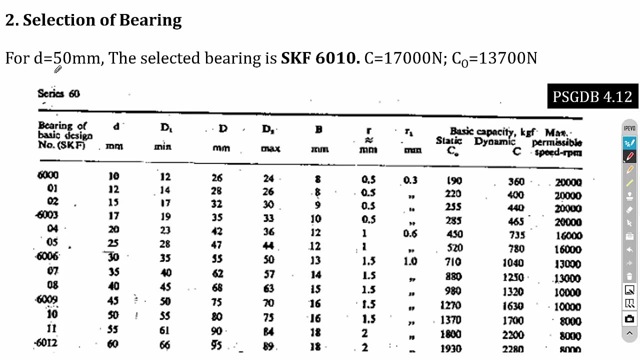 the problems they may give the expected average life. So if the expected average life is given then you have to divide it by 5 to get the expected life. The second step is selection of bearing. So here in the problem the shaft diameter is given as 50 mm, So you can select the bearing. 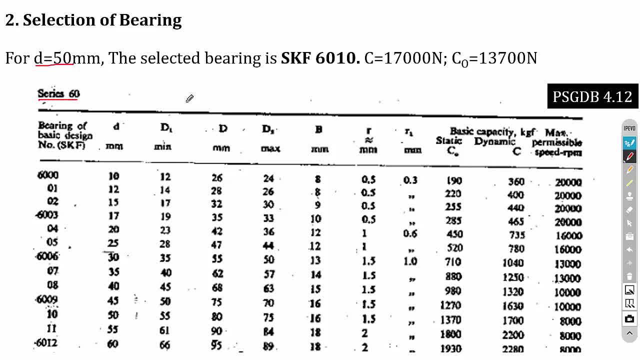 from series 60 or directly you can go to series 62 or 63. So here initially I have started with series 60. So from page number 4.12 from series 60, for a shaft diameter of 50 mm the selected bearing is 6010, and for the selected bearing you can refer that the c value is 1700 kgf. that is. 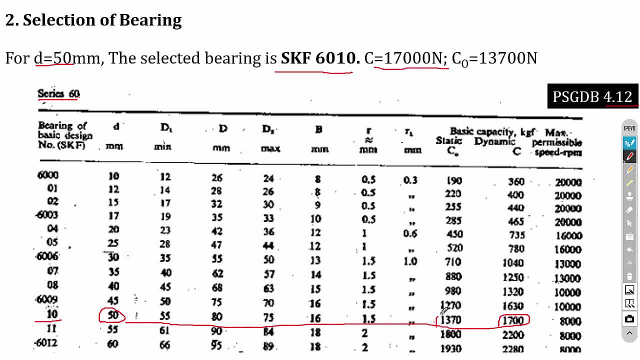 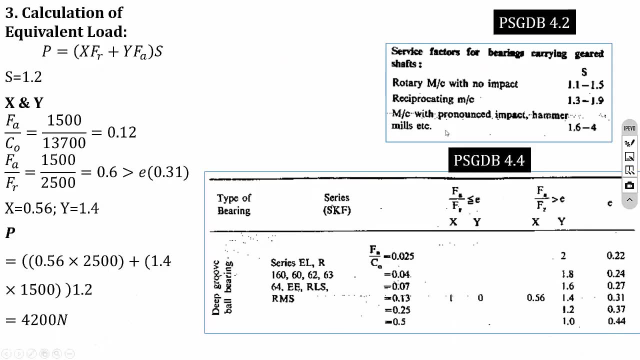 17000 kgf, Then the c0 is 1370 kgf, that is, 13700 N. So now I have selected the bearing that is SKF6010.. Now I have to check whether the selected bearing is suitable for my application or not. For that I 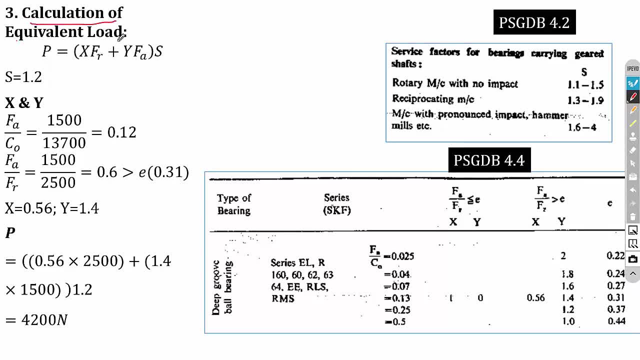 have to calculate the equivalent load. So the third step is calculation of equivalent load. So the equation is: P is equal to X into FR, Then the F is equal to F a plus y into f. F4 is given, f a is given. First we will select the s value, that is service factor. So here it is used for an air compressor with no impact. So you can select the s value in between 1.1 to 1.5. I have selected a s value of 1.2.. 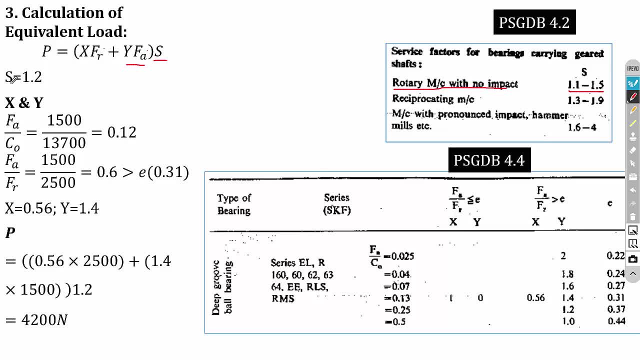 Then the next one is selection of X and Y. So, as I told earlier, to select the X and Y you can have to see the page number and you can see P and Y. So here it will be same as before 4.4. so in that you will have a chart. so i have cropped the chart and i have selected only for. 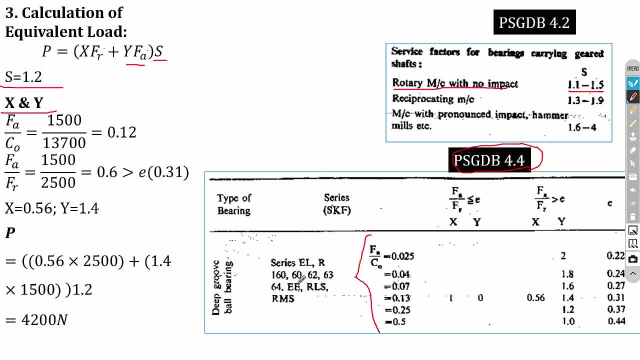 ball bearing, that is deep groove ball bearing. so this is for series 60, 62, 64, 60 el, i mean ee and rls. okay, so here to select the x and y value first i have to calculate the fa by c naught. so fa by c naught is equal to fa is given in the problem, that is, axial load is 1500. 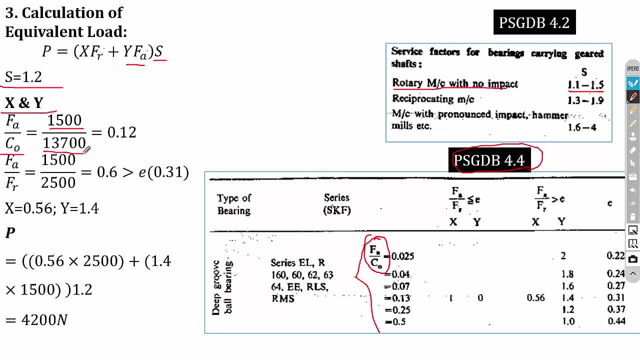 newton and c naught is the static load carrying capacity of the bearing. it is 13700. so this is from the data. so fa by c naught value is 0.12. okay, so you can refer the fa by c naught value. so the next standard value is 0.13. so this is going to be my row of selection. 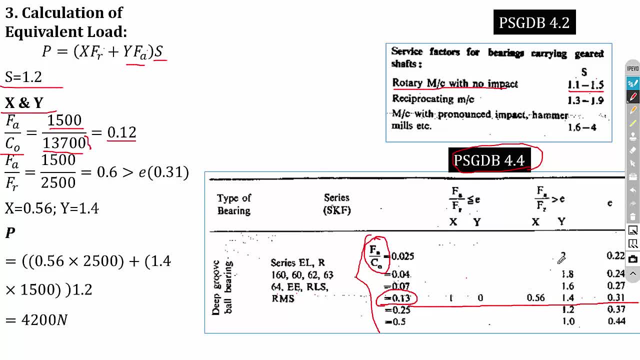 so next i have two xy, x values and two y values. so to select x and y, next is i have to select the fa by fr value. so that is calculation of fa by fr. so fa is 1500 and fr is 2500, it is equal to 0.6. and for fa by c0 is 0.13. the e value is 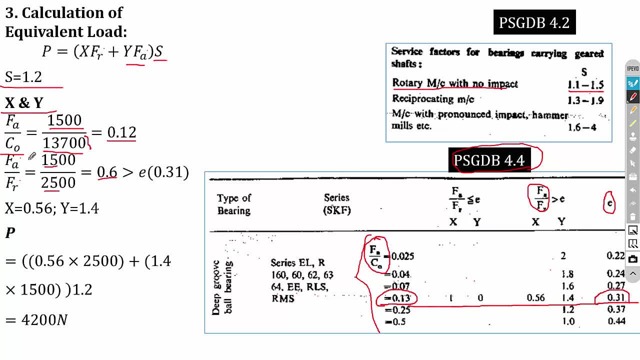 0.31. so the fa by fr value, that is, 0.6, is greater than the e value. so you can refer this column. so your x value is 0.56 and your y value is 1.4. so my x value is 0.56 and y value is. 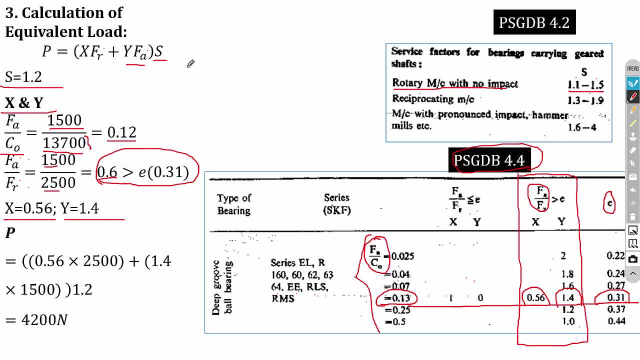 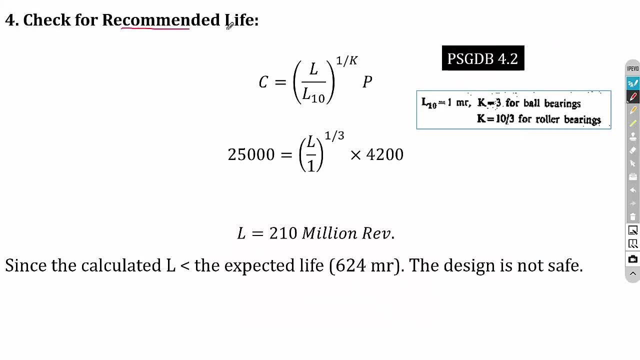 1.4. so now we can substitute everything in the equation and we can calculate the equivalent load. that is 4200 newton. okay, so that is the calculated equivalent load. so the last step is check for recommended life. so to check for recommended life, first i have to calculate the life of the selected bearing. so the 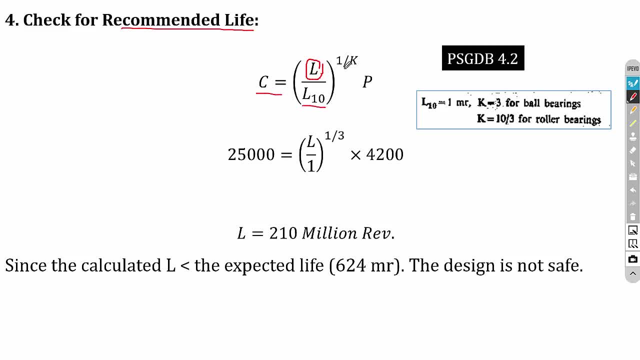 equation is: c is equal to l divided by l 10, whole power, 1 by k into p. okay, so this the equation is there in page number 4.2. you can refer that. so c is the dynamic load carrying capacity. it is from the data book. so first substitute the value of c. l 10 is 1, so for ball bearing k value is equal to. 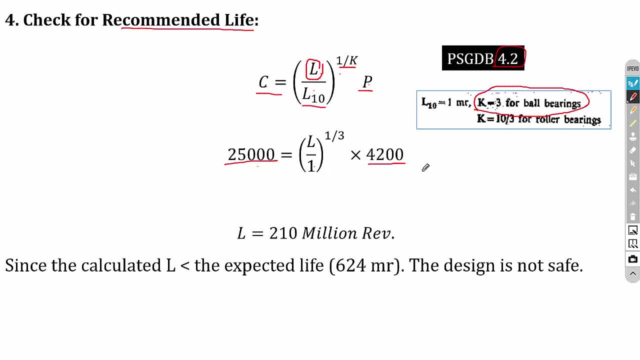 0.3 and p i have calculated that is 4200. so if i solve this equation i will get: l is equal to 210 million revolution. but if you look into the expected life, that is life from the step 1, it is 624 million revolution. so the calculated l is less than the expected l. actually for safe condition. 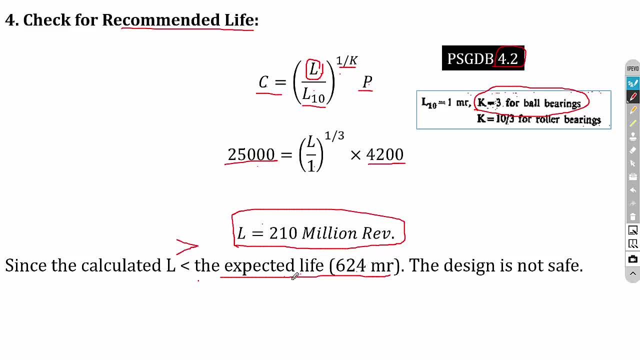 the calculated l should be greater than our expected life. so here it is less than the expected life. so the design is less than the expected life. so here it is less than the expected life. so the the design is not safe. okay, so that is very important. the design is not safe, so i have to. 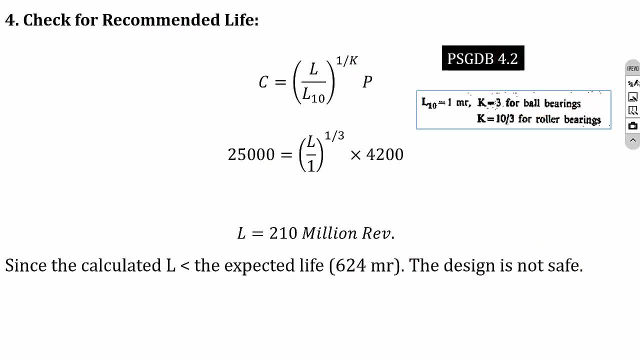 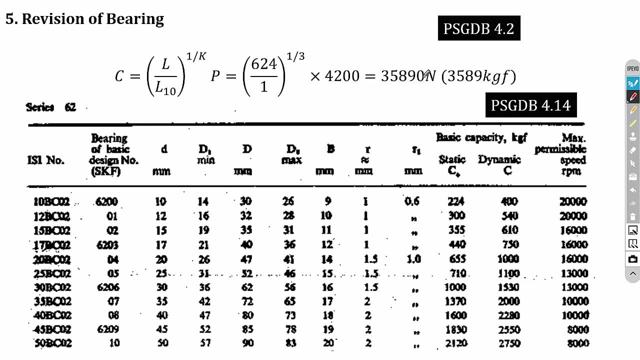 revise the selected bearing so i can move into the step 5. so that is revision of bearing. so if the selected bearing is safe, then you can stop with step 4. so here my selected bearing is not safe, that is why i am moving into the step 5. so the equation is again the same equation, that is: 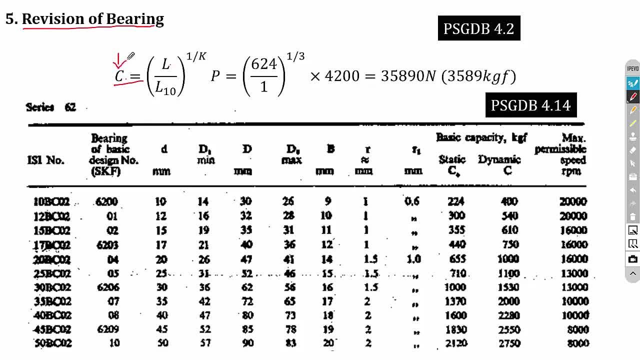 C is equal to. so in the fourth step you have to substitute the value of c and you have to calculate l. in fifth step, you have to substitute l value and you have to calculate the value of c. okay, so l use the l from step 1. that is the expected life. so substitute l, l, 10, k and p. 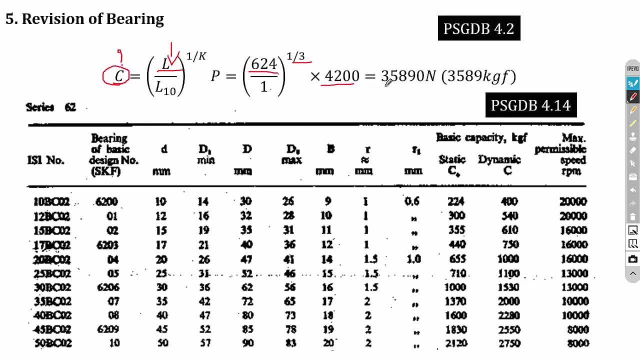 and calculate the value of the c. so the expected c is 35,890 newton. okay, so now welcome, can move into series 62 for 50 mm diameter, because already for series 60 the bearing is failed, so I don't need to go to the series 60 again, so I can. 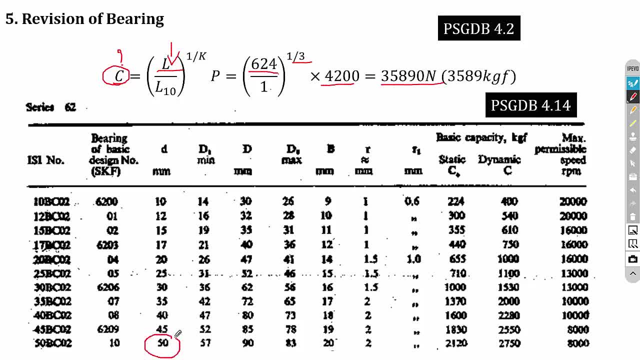 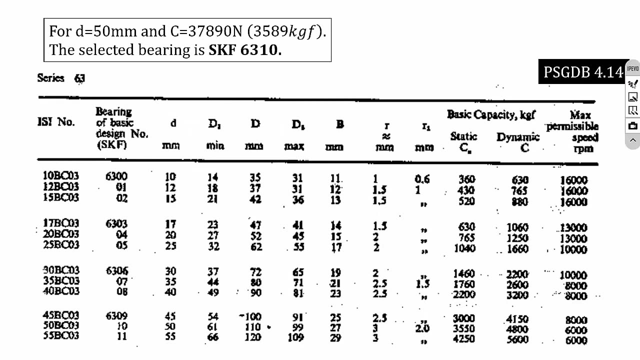 directly go to series 62, for so far 62 and the D is 50 mm. the C value is 2750 kgs, so that is 27,500 Newton, but for my case the expected is 35,000. okay, so the series 62 will not suit for my application. I can move into series 63, so 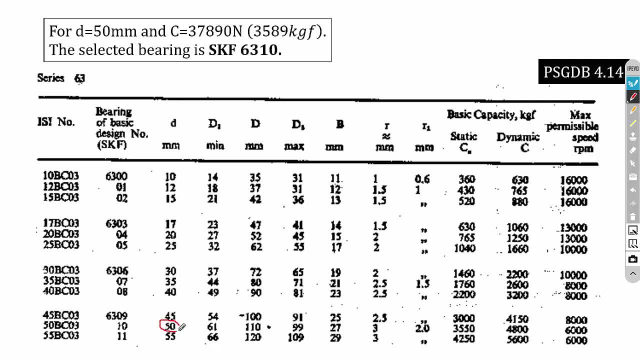 for 63 and 50 mm diameter. the load carrying capacity is 4800 kgf, that is, 48,000 Newton, so it is greater than my expected C value. so this bearing is suitable for my application. and the revised selected bearing is 6310. so the selected 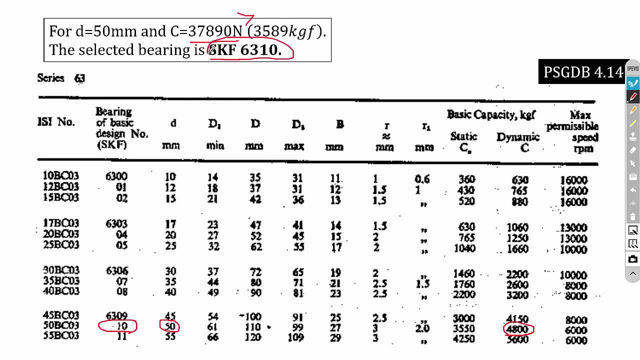 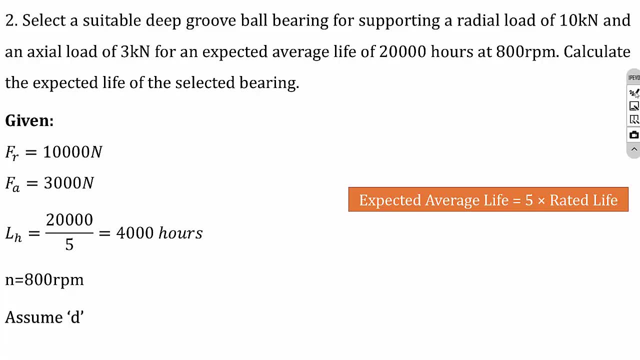 bearing is SKF 6310. okay, so this is how you have to select the bearing. you have to check the recommended life and you have to revise the selected bearing for your application. okay, so the tutorial problem is: select the selected bearing for your application. Select a suitable deep groove ball bearing for supporting a radial load of 10 kN. FR is 10,000 N and an axial load of 3 kN. FA is 3,000 N, for an expected average life of 20,000 hours.